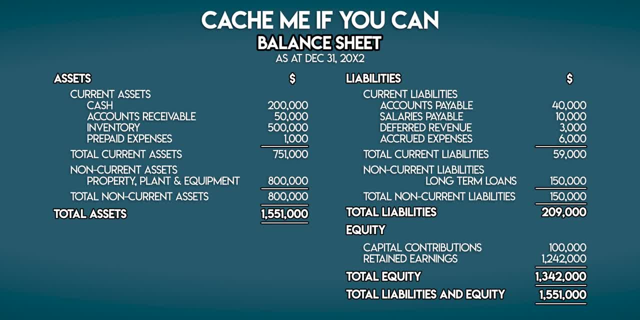 time, then we're looking at a balance sheet. This balance sheet is for a business called Cash Me If You Can, which makes microchips and computer stuff, And what we're looking at is a snapshot of Cash Me If You Can's assets, liabilities and equity at a single point in time. 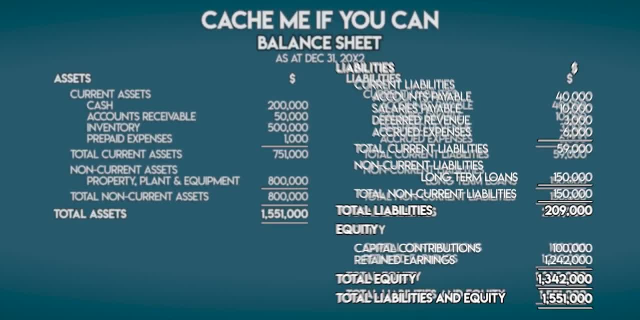 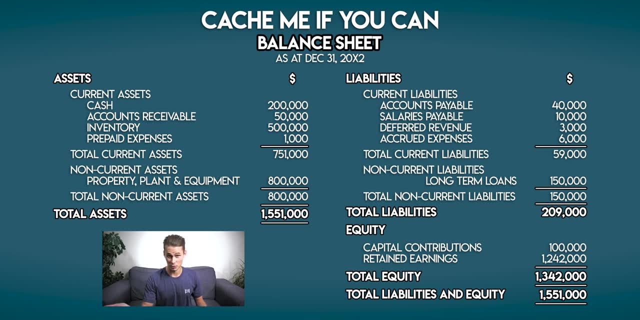 Essentially, it's a summary of what they own and what they owe. on December 31st- Great. But at the start of this video, I said that I'd show you the key to understanding financial statements, And we haven't quite got there yet. Here's the balance sheet, but where's the income? 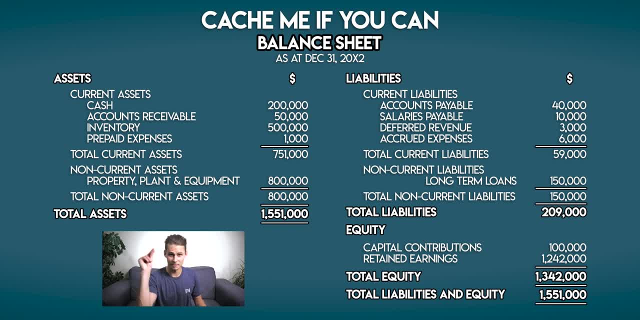 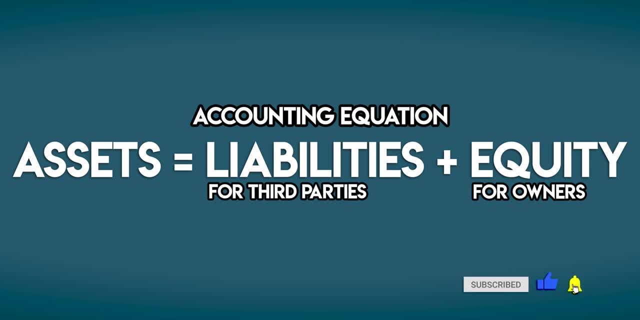 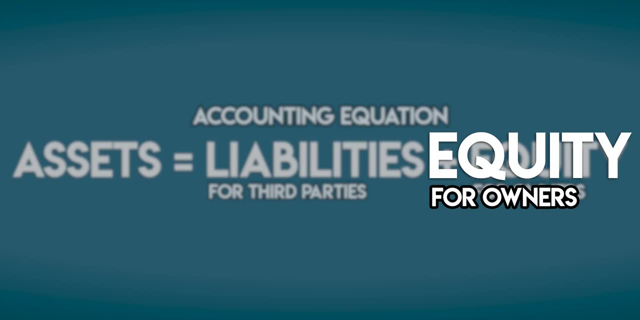 statement. Let's go back to the accounting equation: Assets, equal liabilities plus equity, or the stuff that a business owns is equal to the stuff that it owes to third parties and its owners. But let's focus on equity. What kind of stuff does a business owe to its owners? Two things. 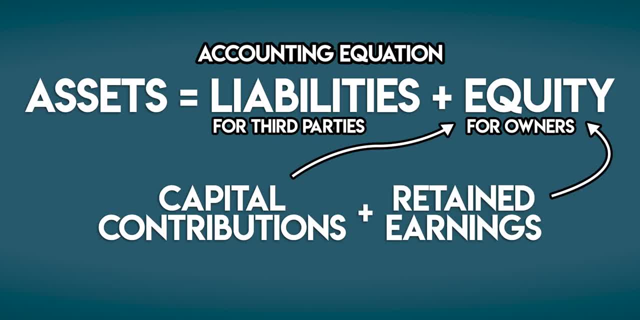 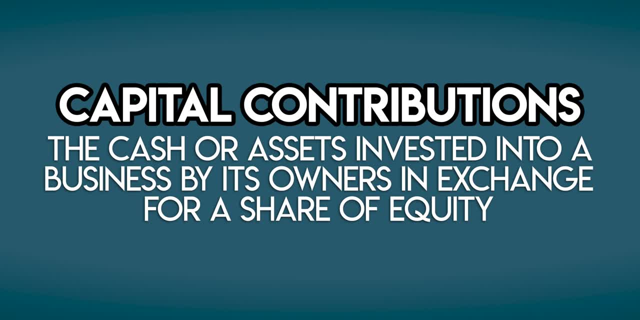 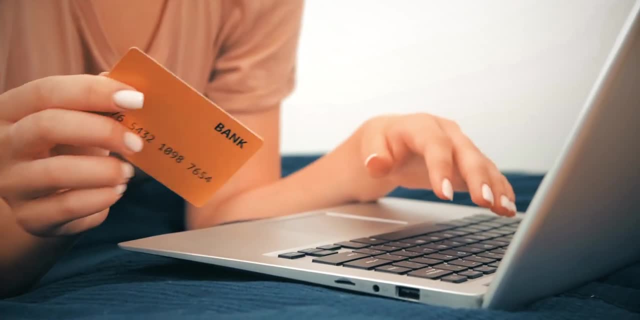 It owes them their capital contributions and the business's retained earnings. Capital contributions is the money that the owners take out of their own pockets and invest in the business. For example, if Cash Me, If You Can issues some shares and you buy one, then you've made a capital contribution. Now you're a shareholder and you're a part owner of. 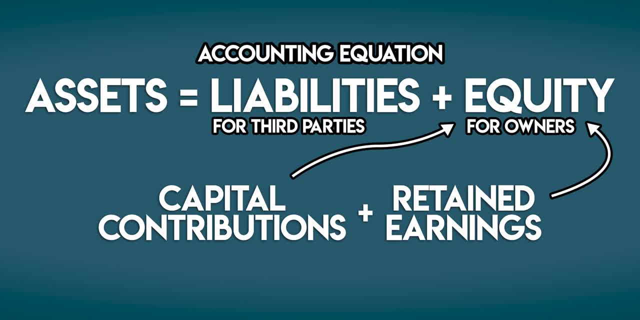 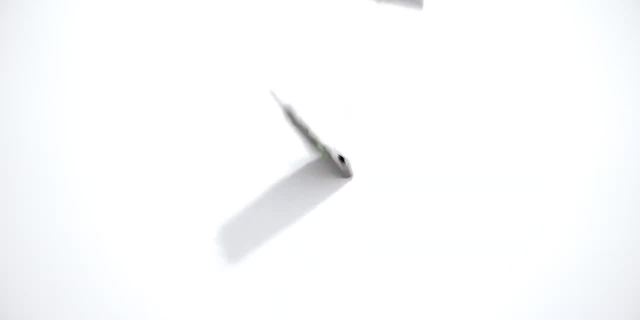 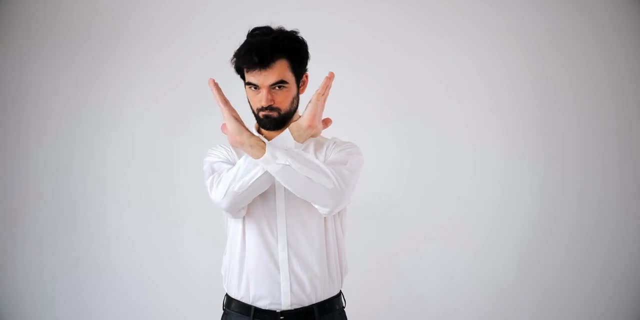 the business. Okay, so what's the deal with retained earnings, then? These are the business's profits that the business is holding onto for the future, And this doesn't mean a huge pile of cash that just keeps on getting bigger and bigger. Cash and profit are two very different things. 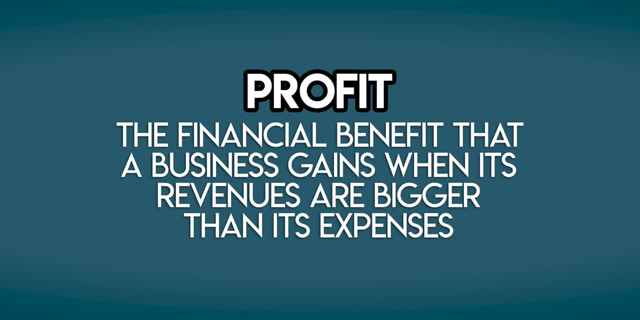 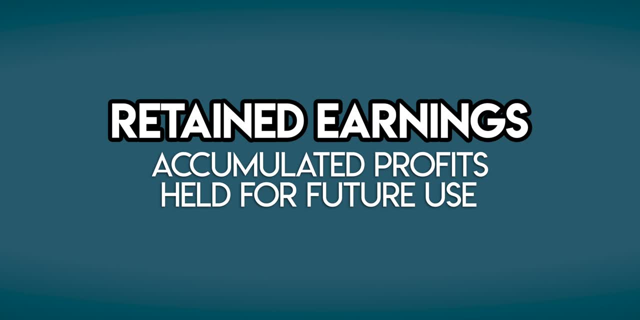 Profit is the financial benefit that a business gains when its revenues are bigger than its expenses, And a business's accumulated profits held for future use is called its retained earnings. This is what's left over after we add up all of the profits that the business has generated. 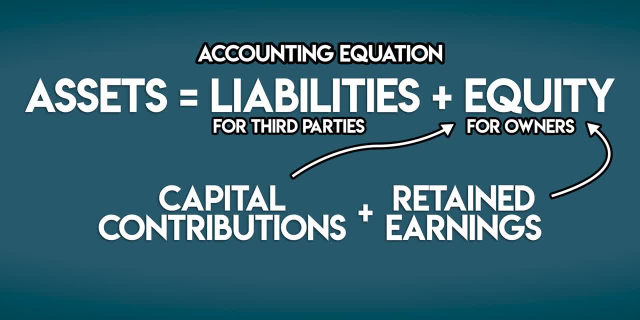 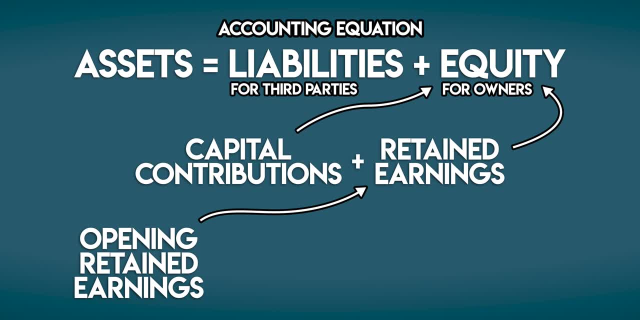 over the years And that looks a little something like this: Retained earnings are made up of opening retained earnings, which is last year's retained earnings carried forward into the start of this year, plus current year profits, which is the difference between revenues and expenses. 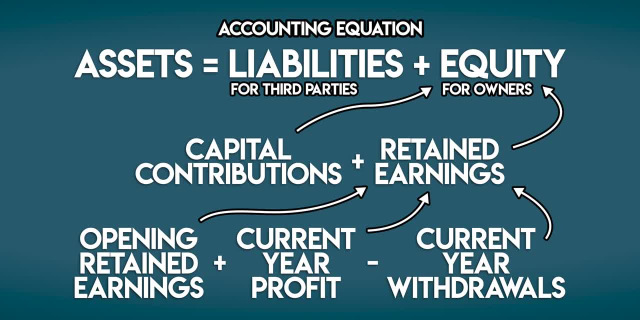 minus current year withdrawals, the profit distributions to the owners or shareholders of the business, which I'm pretty sure you've heard of. We often call them dividends. I like to think of this as the expanded accounting equation And in my opinion it's the key to understanding financial statements. 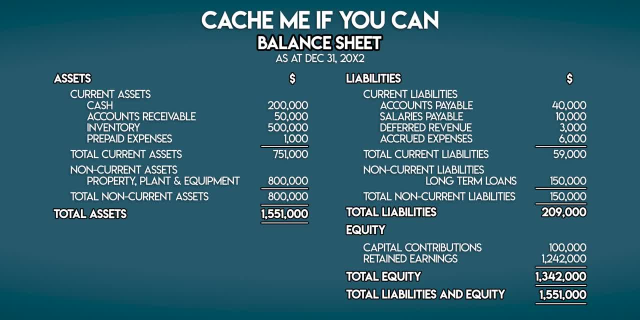 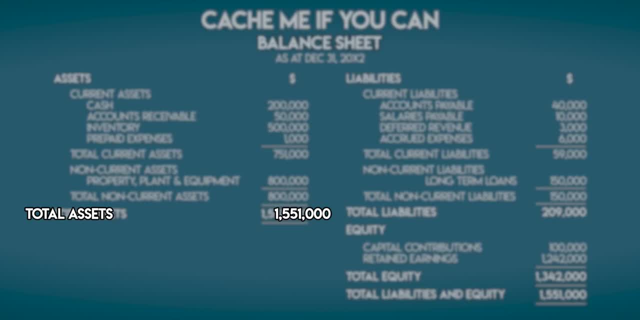 Let me show you why. If we jump back into CashMiffyCann's balance sheet, we can see what the business owns and what it owes. on December 31st, They own $1,551,000 in assets and the same amount in liabilities and equity. 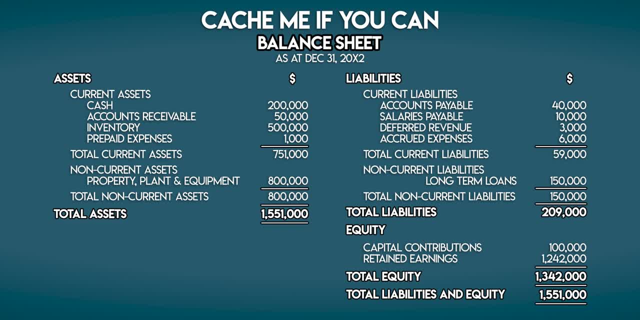 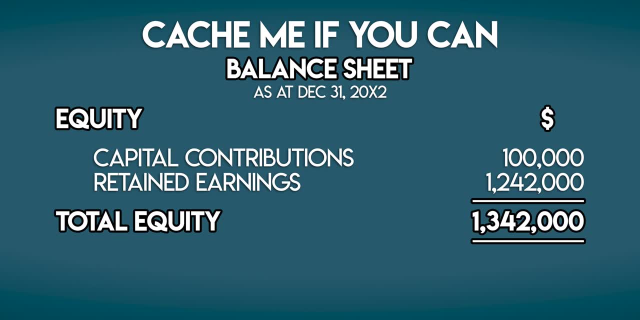 because these two sides of the balance sheet are in balance. Now, if we zoom into the equity section, we can see that CashMiffyCann owes $1,342,000 to the owners of the business, its shareholders, of which $100,000 is made up of capital contributions. 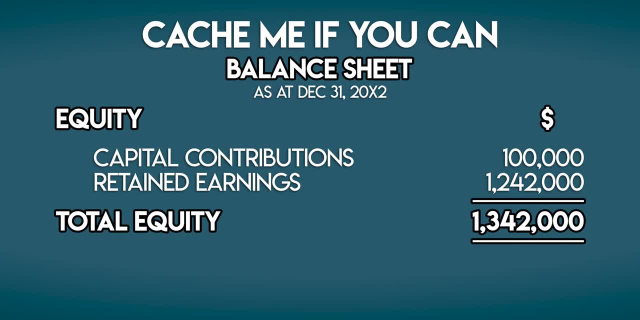 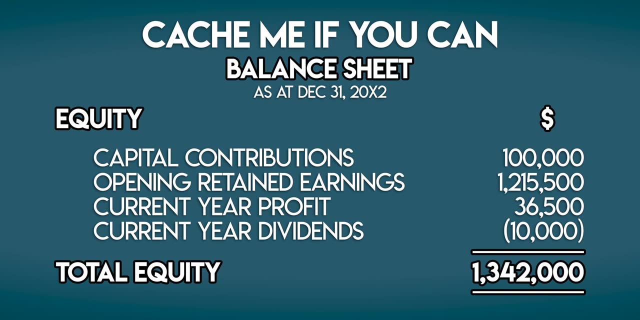 that the owners have put into the business and $1,242,000 in retained earnings. Now here's where things get interesting. If we expand retained earnings, the savings will be brought into FOME BUDGET. we can see what they're made of Last year's retained earnings, which came to $1,215,500. 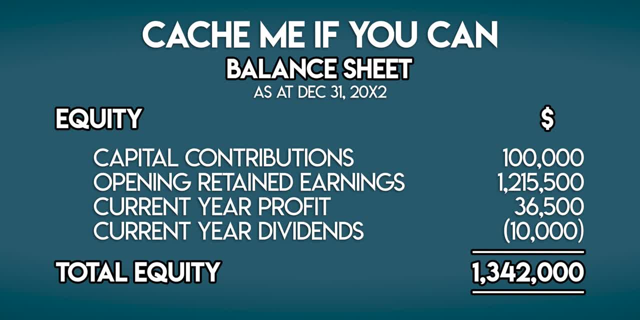 less the current year dividends, which were $10,000.. This number is negative because these profits have been withdrawn by the shareholders and we can also see that this year- Cash Me If You Can- generated $36,500 in profit. Where did they get this number from Current year profit. 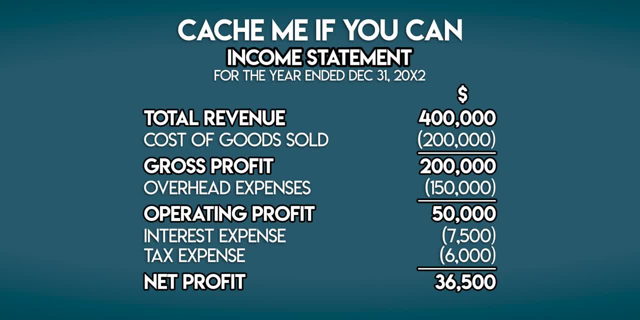 comes straight from the income statement, which looks like this: The income statement summarizes a business's revenues and expenses over a period of time. It's financial statement just like the balance sheet, but this one tracks Cash Me If You Can's performance over a one-year period. 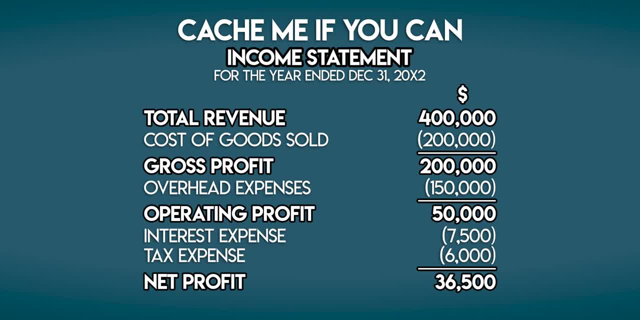 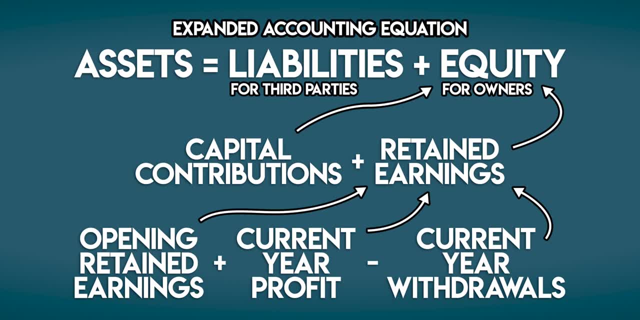 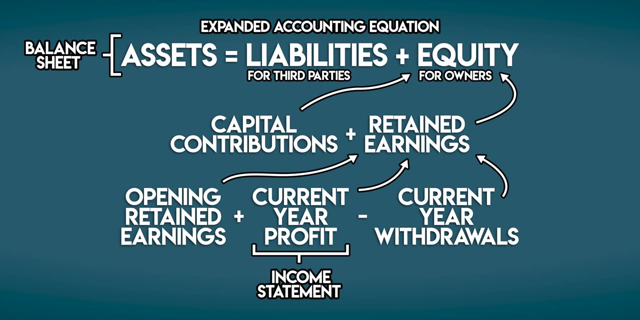 and tells us how profitable they are. Pretty cool, hey. So if you go back to the accounting equation and expand it out, we can see that retained earnings is the key that links together two of the most important financial statements: The income statement and the balance sheet. Thanks to all my channel members for supporting Accounting Stuff. Your